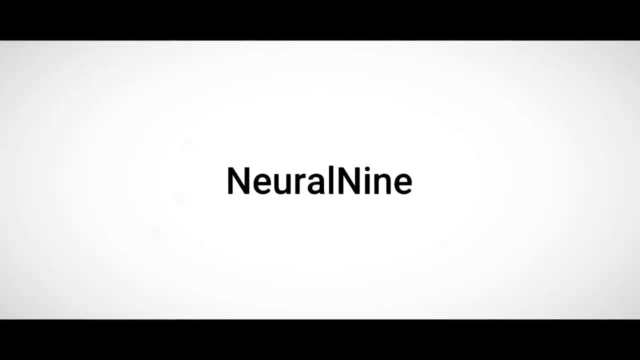 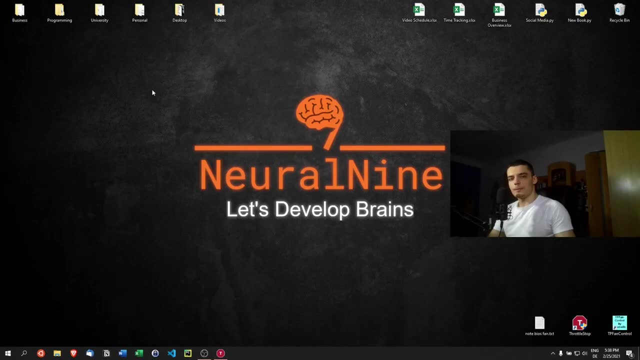 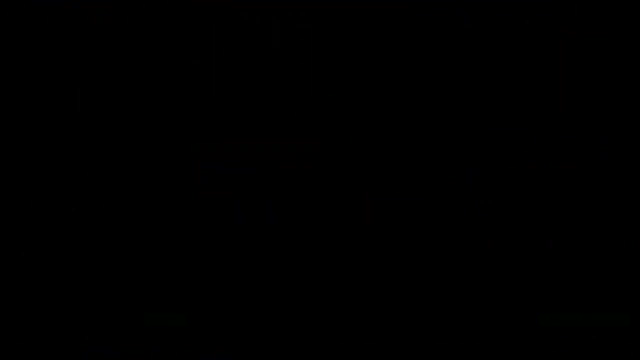 What is going on, guys? Welcome back to the advanced Python tutorial series. In today's video, we're going to talk about the singleton design pattern, So let us get right into it. Alright, so you guys really seem to enjoy those design pattern videos, So today we're going to 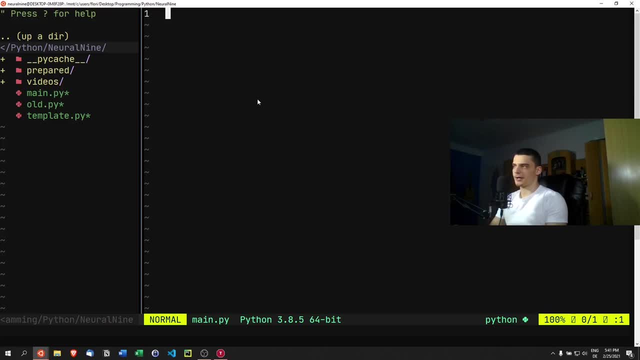 talk about another one, And the singleton design pattern is actually quite simple. The basic idea is that we have a class and this class can only have one single instance. So if we have, for example, a class person, a normal class person, we can do as many person objects as we can fit into. 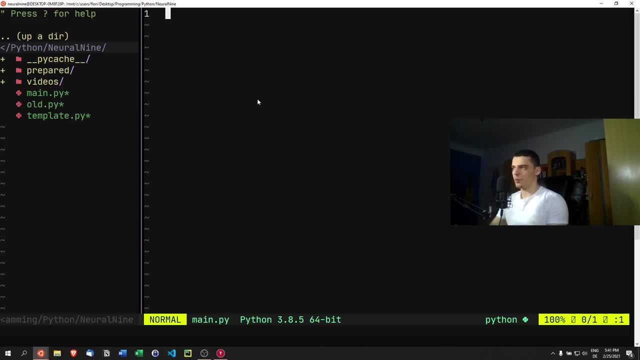 the memory, Whereas in a singleton we can only have one person, one person object, that person would be a singleton. So this is what we're going to model today: We're going to again import from ABC, So from abstract class, we're going to import ABC meta And we're going to import. 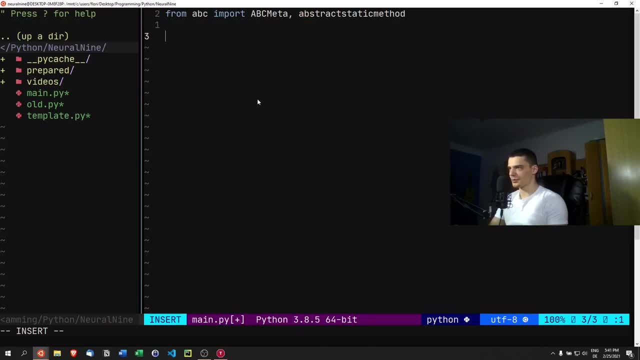 abstract static method, Because we're going to work with an interface just for the sake of it. we're going to have an interface person, So I person, and the meta class is going to be going to be ABC meta. There you go, And we're going to have one method in here. 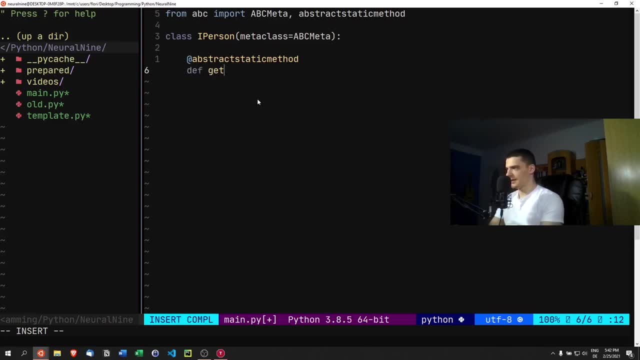 which is going to be an abstract static method, And this is going to be get data of this person And we're going to implement it in the child. So implement in child class, like that, And then we can have a person singleton class. So we're going. 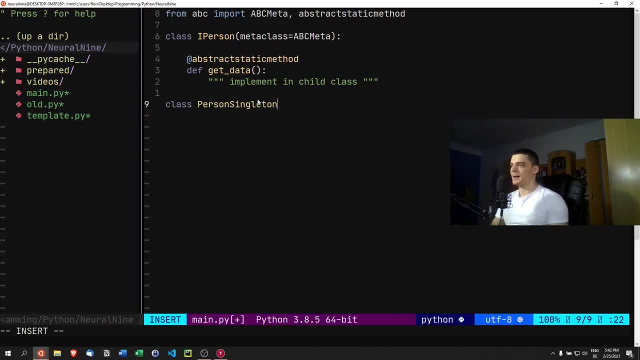 to say class person singleton. And, by the way, I just want to mention here that this is not the only possible implementation. you can do many different things. you can use decorators, you can use your own meta class, you can have an interface I person and also a class singleton that you 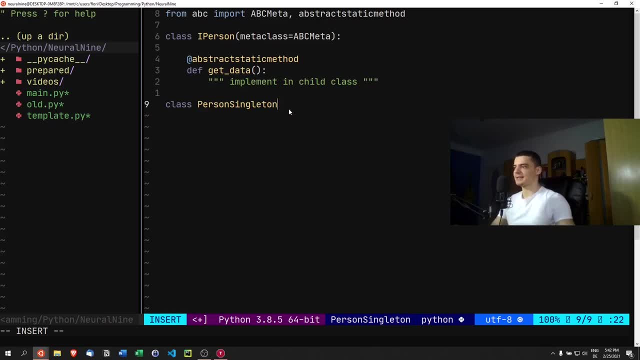 extend or inherit in the in the person class And then we're going to have a person singleton. So there are many ways to go about that. I think there's a stack overflow question where one guy asked how to do a singleton design pattern in Python And the top answer had like four methods. 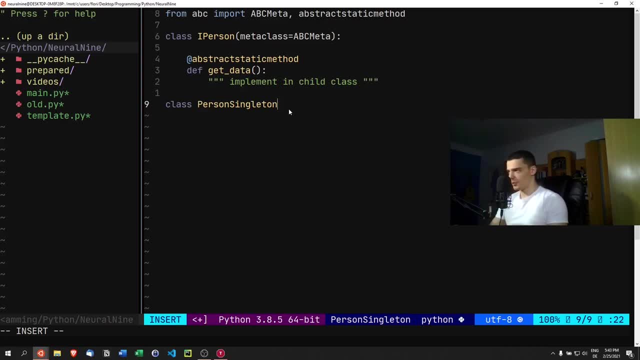 so you can use all of those, But this is just one of them or one possible way to implement a singleton design pattern in Python. So we're going to extend from the or inherit from the I person interface And in here we're going to say, instance with two double underscores, or actually. 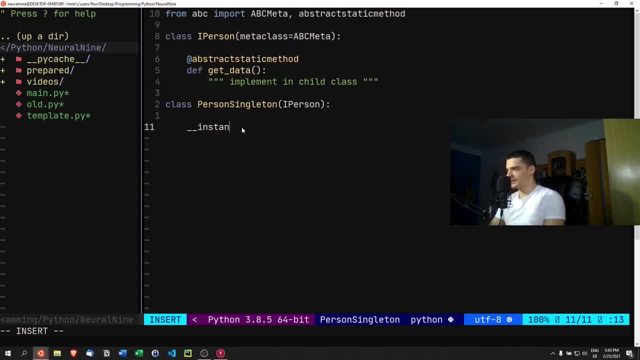 yeah, with two underscores before the name, so that it's private and we're going to say: instance is none by default. So this is this instance thing here. this instance variable is going to be the one, the single one instance that we can create here, And what we're going to do then is we're 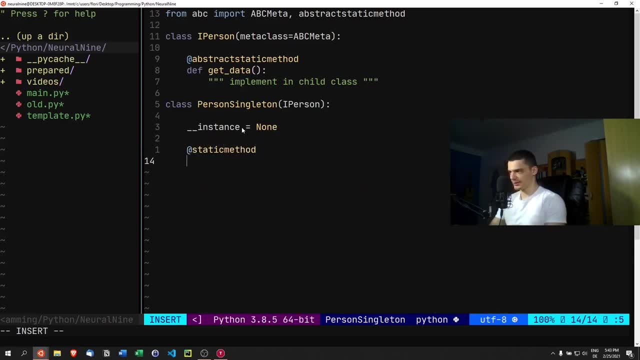 going to have a method called static methods, or it's going to be a static method and it's going to be called get instance, So we can get the current instance, or actually the only instance that there is, And what. we're going to be able to polymerize that, since in this case, we're just going. undeleted or we'll leave it undeleted. But with respect to the сегодня's votes, we're going to need to apply to a specific instance calledAB lever on here and a, because we want to show them that in general, 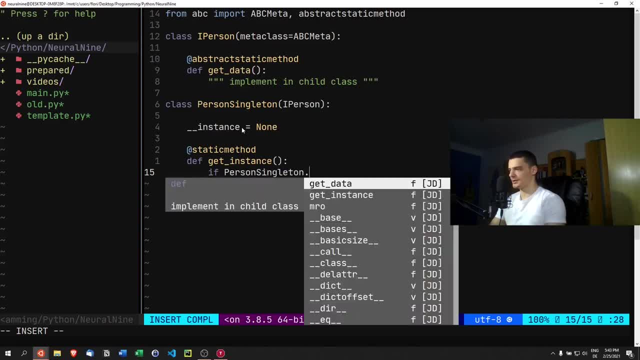 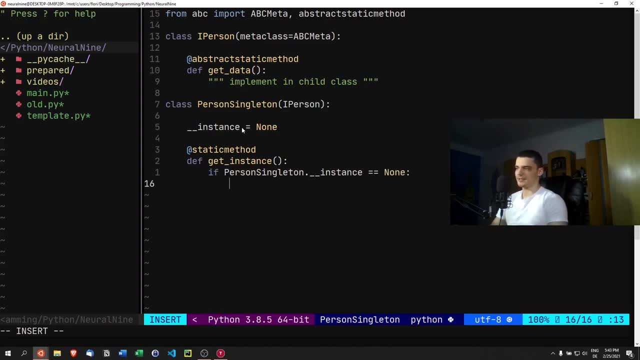 to do here is we're going to say, if person singleton dot instance, if this instance equals none, now here we can do different things. Now this is basically the case where you're requesting the instance, But no instance is there. So we haven't created a person object yet, So there's. 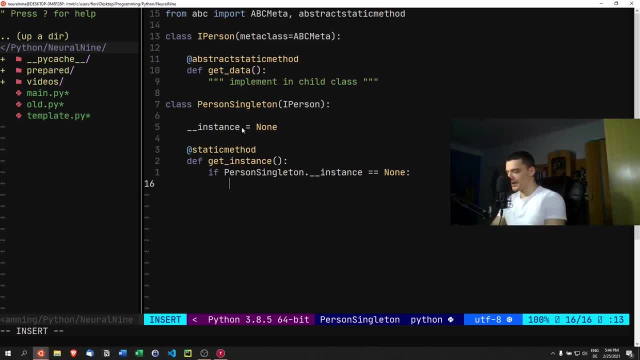 not even a single instance. Now, here you can. one way is to just say, and is to say something like print error because there was no instance found. or you can just create one. Now, of course, if you have some parameters, you can, you can enter some default values and then later on change them. 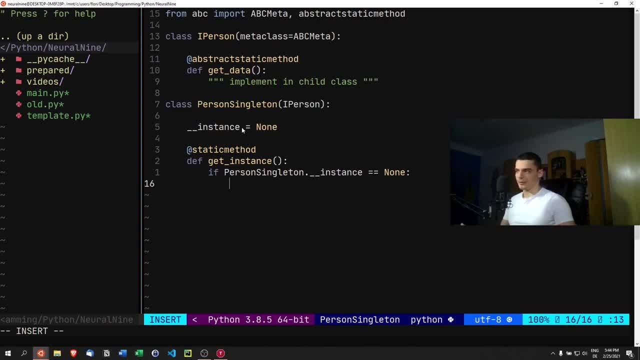 But that's up to you. Maybe you don't want to to allow to get an instance here because you say, okay, there is no instance, I'm not going to return anything, or you're going to return none. that's also possibility. In this case, we're just going to create a person, singleton. 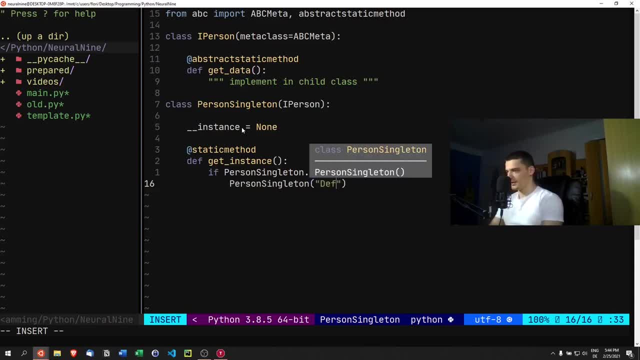 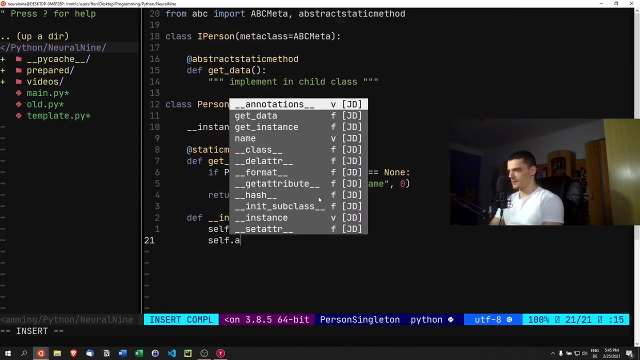 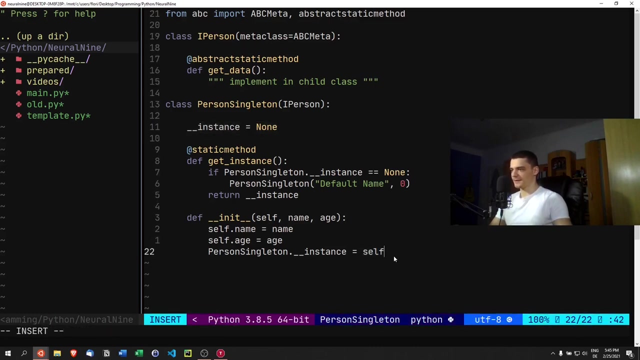 with a default name- we can choose whatever we want for that name- and a default age of zero, And if and person singleton instance equals self, so that this instance here gets the object self assigned. Now, one thing that we need to add here, though, is that we need to make sure that this: 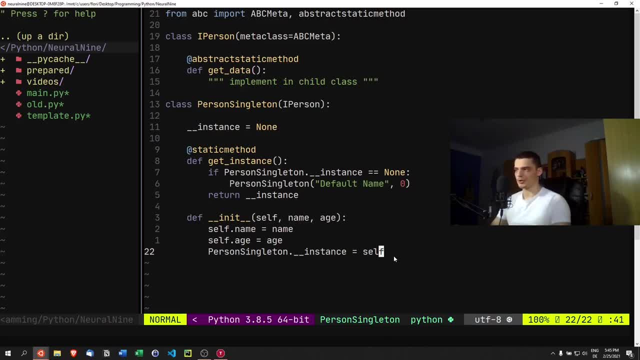 constructor cannot be used multiple times, because then we would always override the instance. And for this we're going to add a simple if statement. So we're going to say: if person, singleton, instance, instance, it's not none, So if we already have one, we're just going to do nothing. I mean here again: 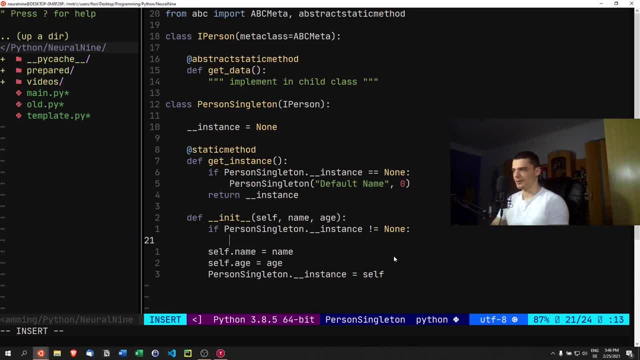 we can choose. what do we want to do? we can do nothing, So we can just skip the constructor. we can say, okay, there is already an object and do nothing. Or we can even raise an exception and say, okay, we're not just going to tell you that there already is an instance, we're also going to 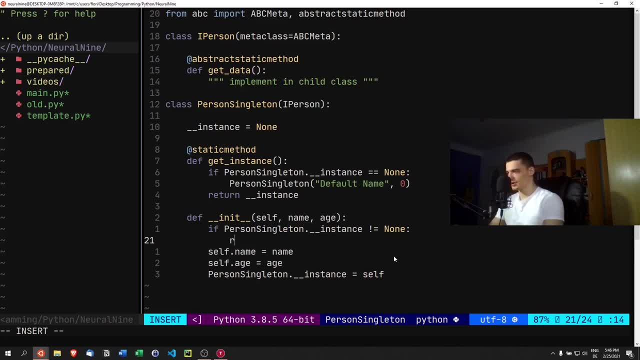 raise an exception and create a problem for you so that you need to catch that. So we're going to add theprofile And then we're going to say, OK, we've created a wow moment state in that We have a throw event. 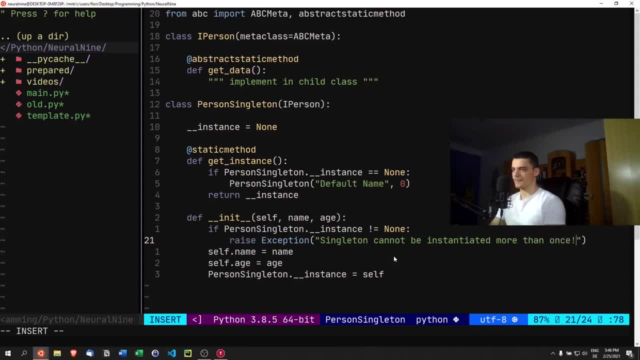 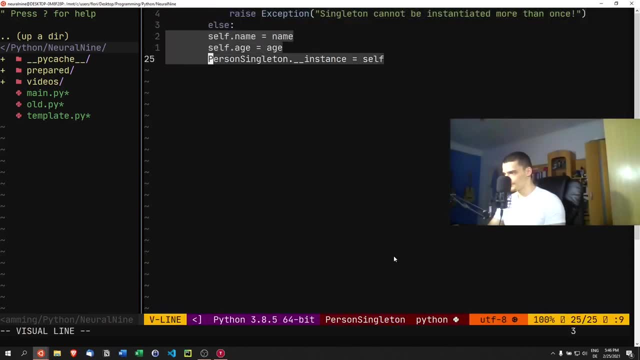 I'm going to clear that we're going to tick it off. I'm going to make a calender, I'm going to let it be. Let's say like this: Because we have our function type in here, we're just going to hand it over. 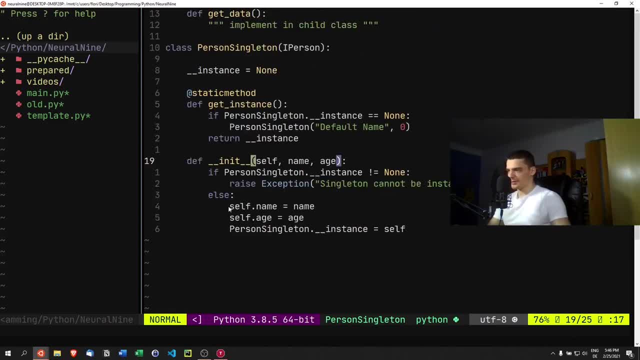 primarily to others. ribbon, we're just going to create, to assign the values and to assign the self object to the instance. So this is the basic way in which we create an object, And then we're also going to have to implement the extra abstract method, which is get data, And in this case this is quite simple. 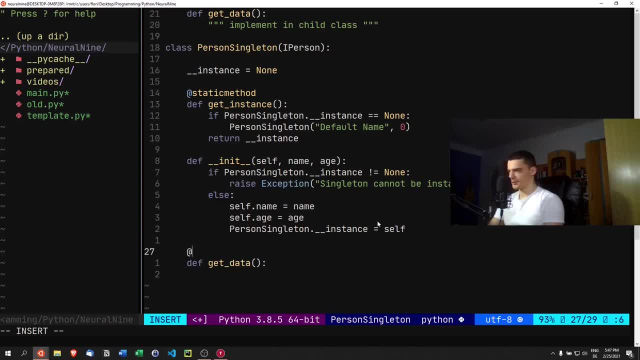 we're just going to. since it's a static method, we need to add the annotation here. we're just going to get the data from the instance So we can say something like: um, actually did we call it get data. let's rename it to print data, because get is most of. 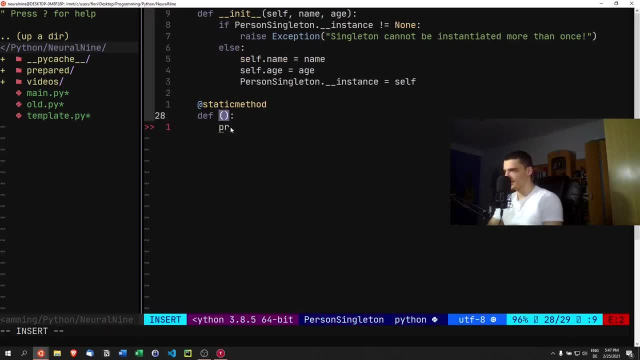 the time a return thing and print is printing, obviously. So we're going to call it print data, And then we're going to just print a formatted string in which we say name is person, singleton, instance, name, like that, And then we're going to do the same thing for the age. 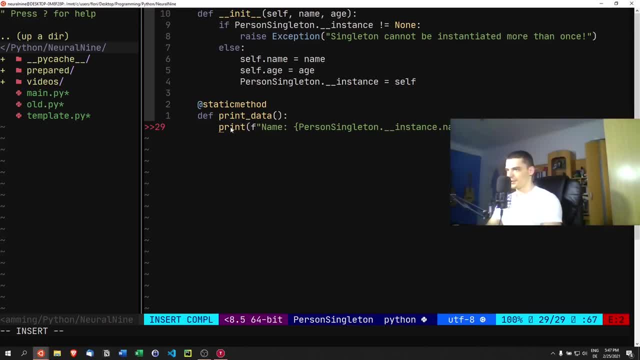 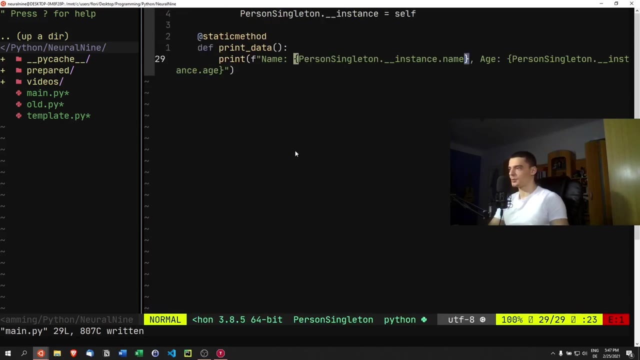 So we're going to say: age is person, singleton, dot, instance, dot h. So that's it. And then what we can do now is we can create, or we can try to create, more than one object and we're going to see what happens. But first of all let's do it in a proper way here. 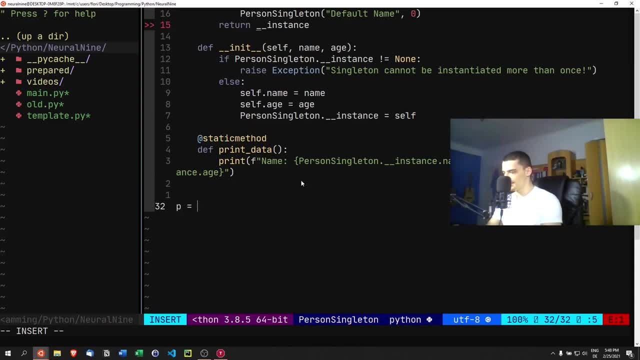 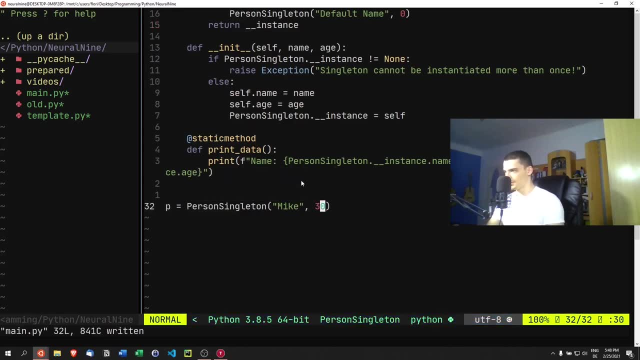 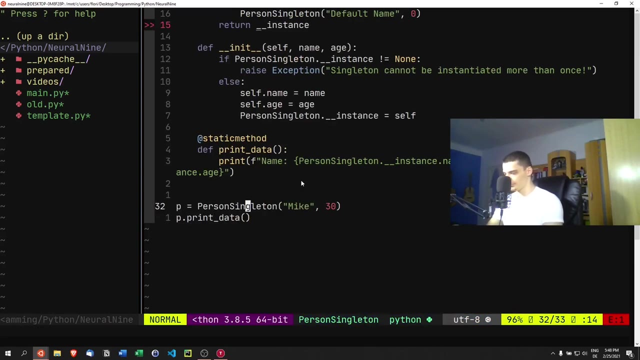 So let's just go ahead and say, I don't know, p equals person singleton, And let's add the name Mike, and Mike is 30 years old. And then we can go ahead and say p dot print data, And we can also go ahead and print p as an. 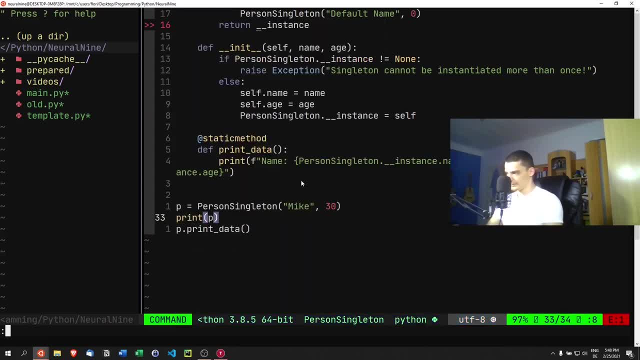 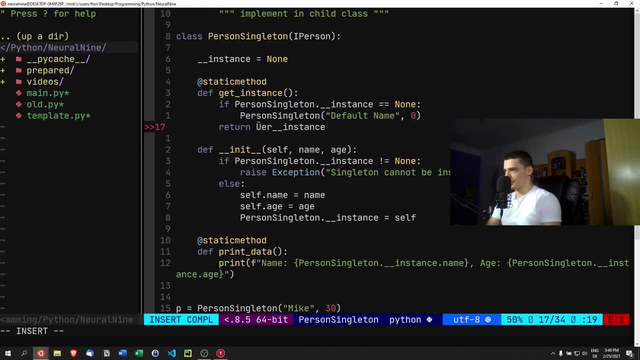 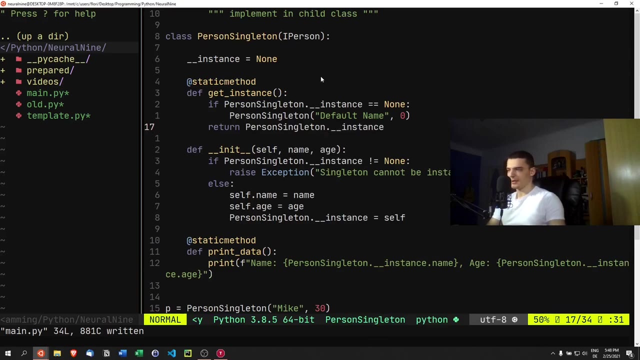 object. This is going to be important for later on. Now let's see if we have any errors. doesn't seem like that. Oh, we have one. Okay, we need to return the person person singleton dot instance. That should be it. Yes, So then we can open up a terminal here. terminal split dash. 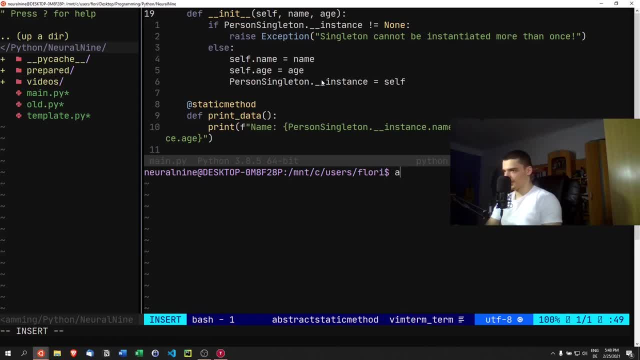 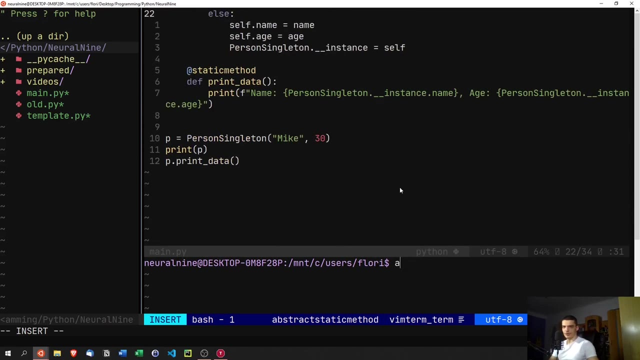 and we can navigate to the. I hope I'm not blocking, by the way, with the camera I bet I'm blocking everything again. So let me just resize this here. Let me go through the code again so that you guys don't have to complain in the comment section. So this is the code. There you go And now. 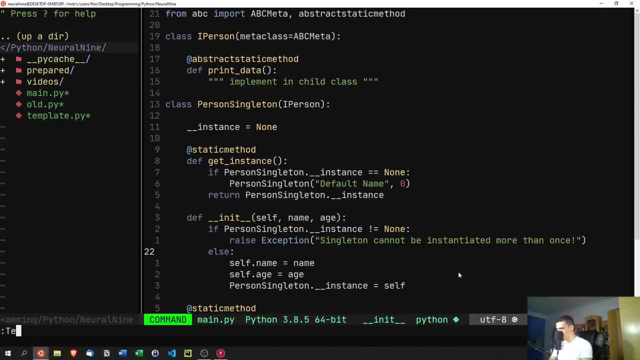 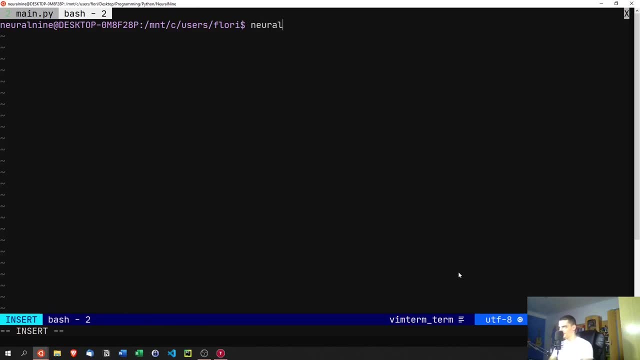 actually let's go ahead and open this in a new tab here. So let's say terminal, tap, bash, And now we're going to navigate to this directory And we're going to say Python three main dot py, And you can see we have this person: singleton.